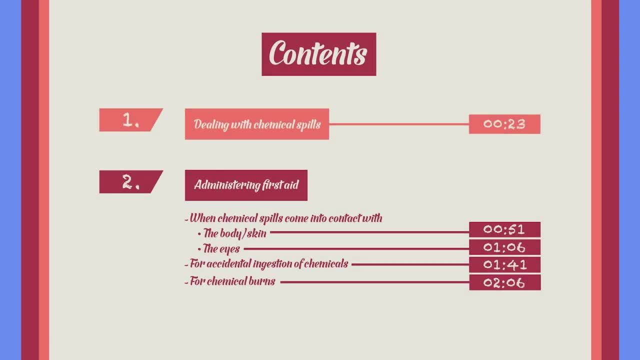 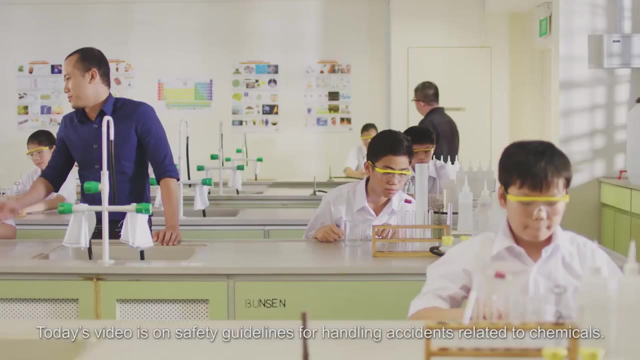 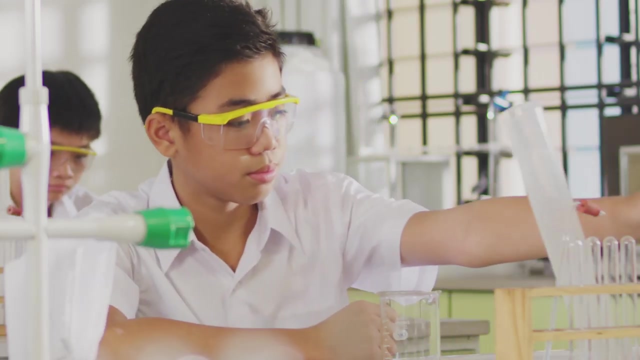 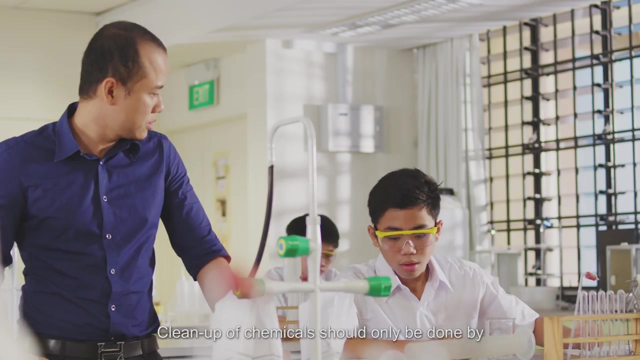 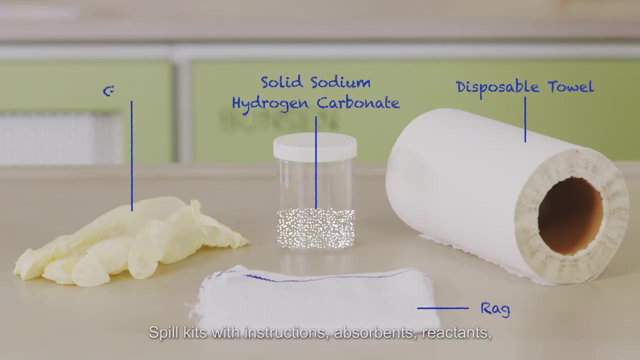 Today's video is on Safety Guidelines for handling accidents related to chemicals. In the situation of chemical spills, inform a teacher or a laboratory staff immediately. Cleanup of chemicals should only be done by knowledgeable and experienced teachers or laboratory staff. Spill kits with instructions, absorbents, reactants and protective equipment should. 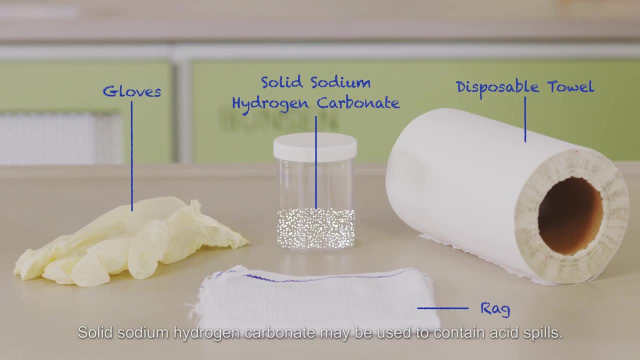 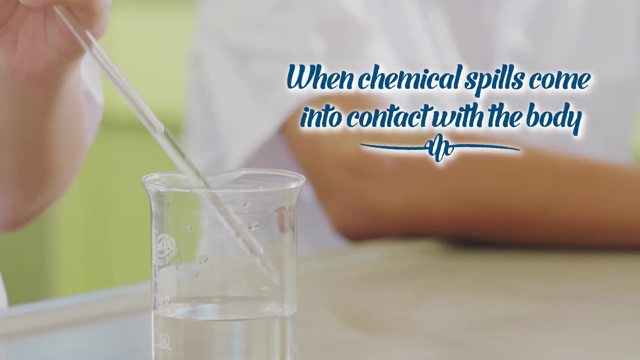 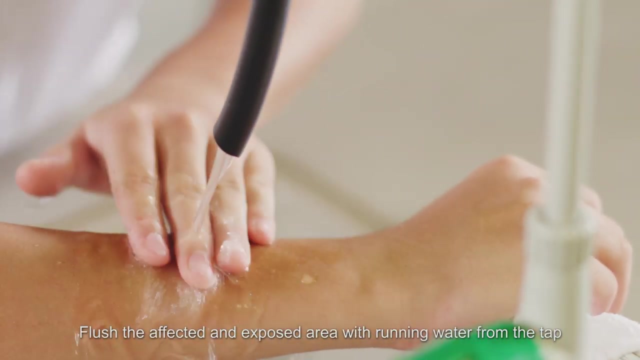 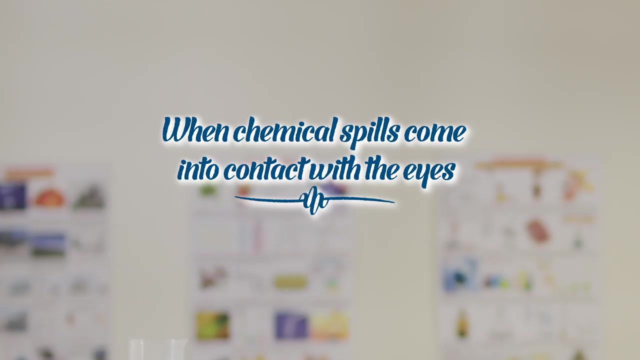 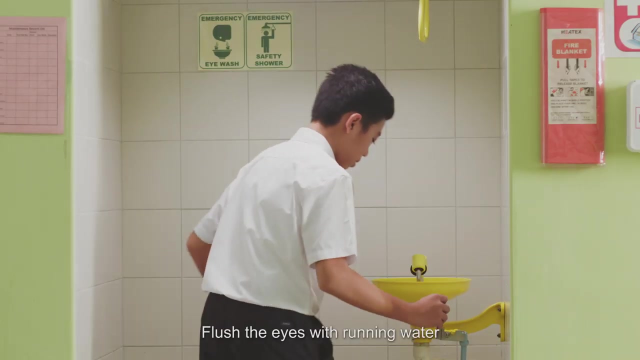 be available to clean up minor spills. Solid sodium hydrogen carbonate may be used to contain acid spills. Flush the affected and exposed area with running water from the tap or safety shower for at least 15 minutes. Remove contaminated clothing. Flush the eyes with running water using the eye washers in the laboratory for a minimum. 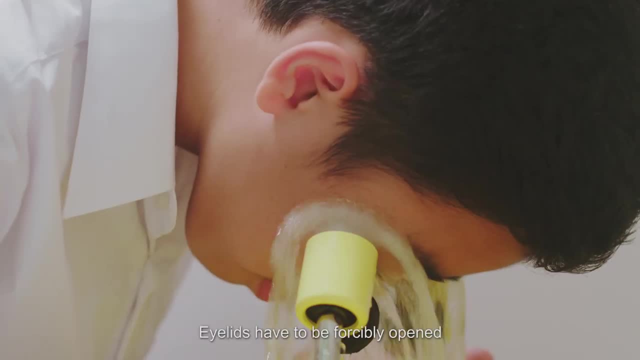 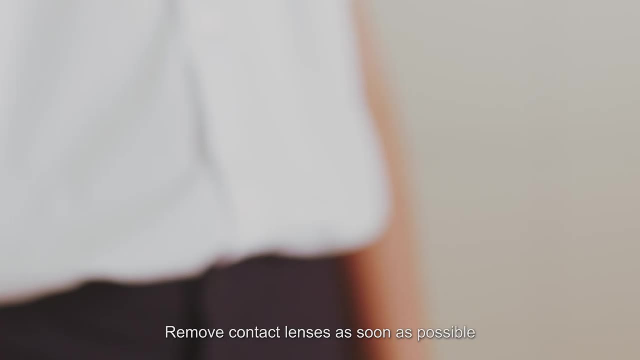 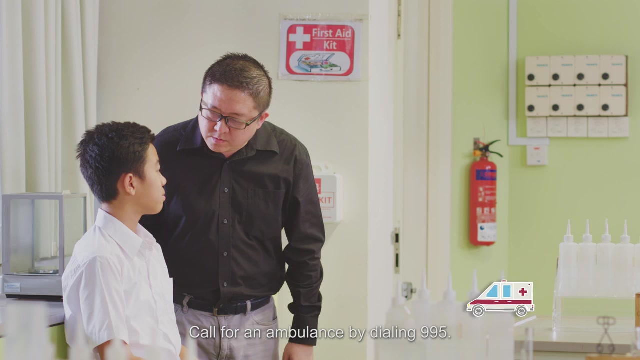 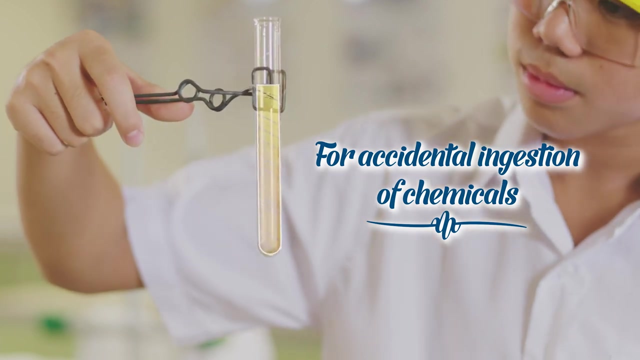 of 15 minutes. Eyelids have to be forcibly opened To ensure that the water or eye solution goes behind the eyelids. Remove contact lenses as soon as possible in order to rinse off any harmful chemical from the eyes. Call for an ambulance by dialing 995.. 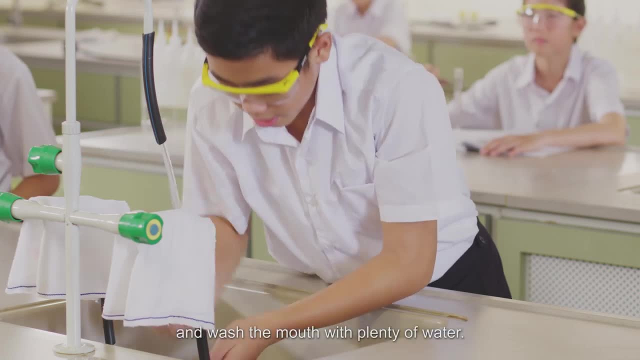 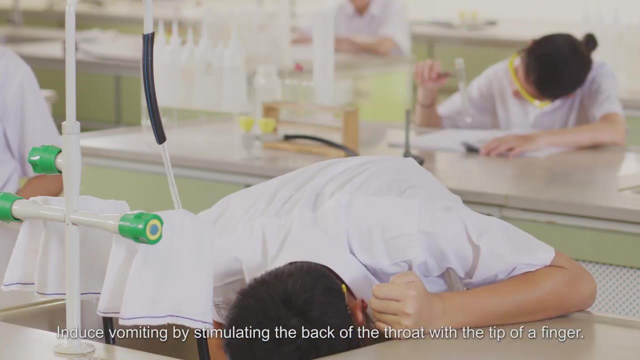 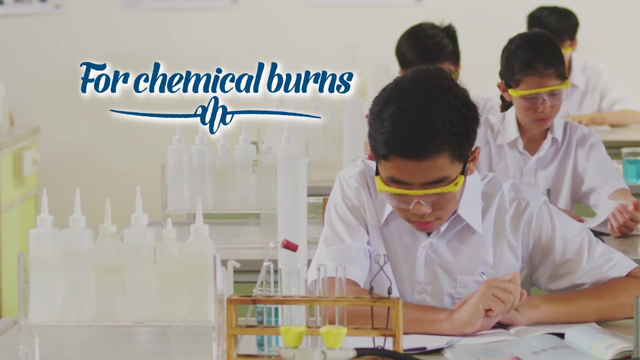 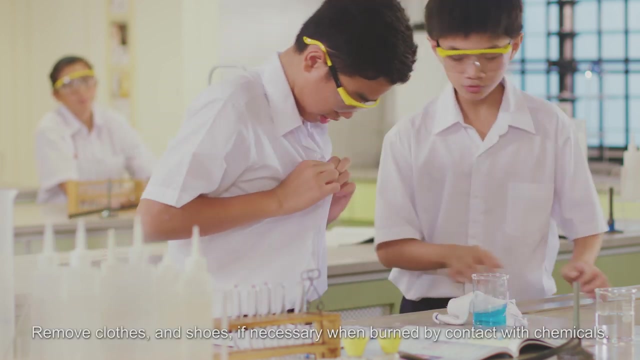 Spit the chemical out if it is still in the mouth and wash the mouth with plenty of water. Induce vomiting by stimulating the back of the throat with the tip of a finger. Seek medical attention immediately. Remove clothes and shoes if necessary when burned by contact with chemicals. 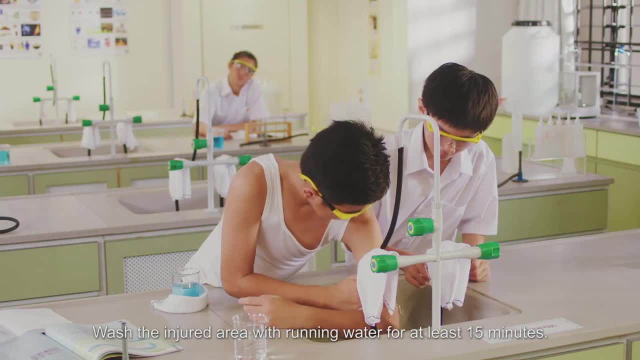 Use water for treating chemical burns. Wash the injured area with running water for at least 15 minutes To remove contaminated clothes and shoes, if necessary. when burned by contact with chemicals, Use water for treating chemical burns. Wash the injured area with running water for at least 15 minutes. To remove contaminated clothes and shoes, if necessary, when burned by contact with chemicals. Use water for treating chemical burns. Wash the injured area with running water for at least 15 minutes To remove contaminated clothes and shoes, if necessary when burned by contact with chemicals.